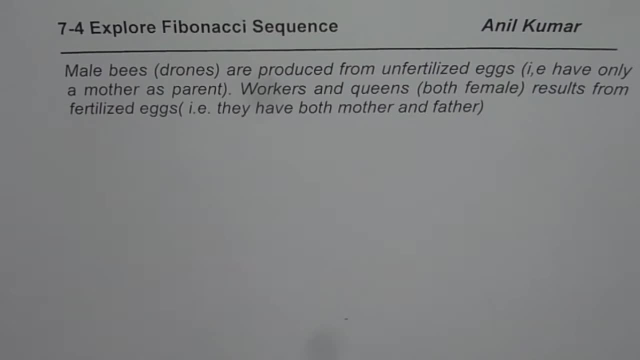 I'm Anil Kumar, and in this video we will explore more about Fibonacci sequence. Now, reproduction of rabbits is a very familiar question here, But working with bees is kind of not so popular, So we will explore more about bees in this particular example. 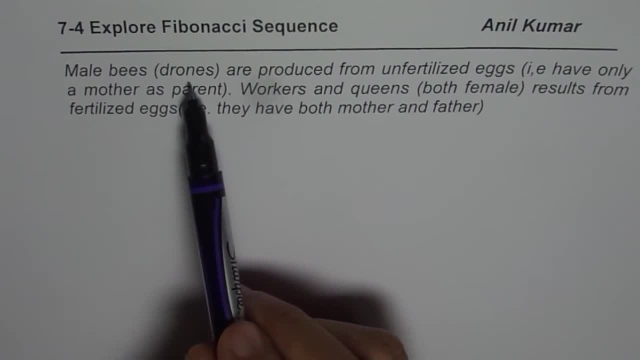 So, as you know, male bees, which are drones, are produced from unfertilized eggs. That means they have only mother as their parent. However, the worker and the queen bees, which are both female, results from fertilized eggs. That means they have both mother and father. 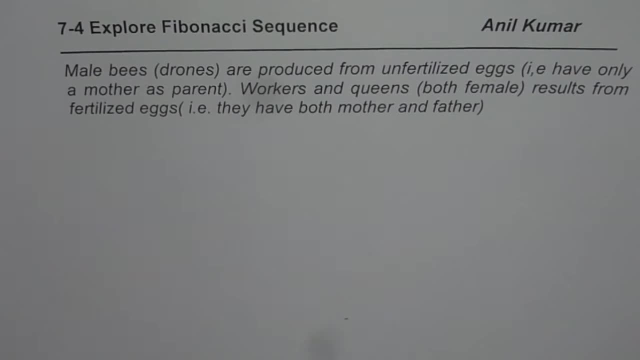 Now, if I have to make a tree, a family tree for a drone, then how is it going to look like? So you can just pause the video and sketch a family tree for a drone and see what you get. Do you get something like a Fibonacci sequence? 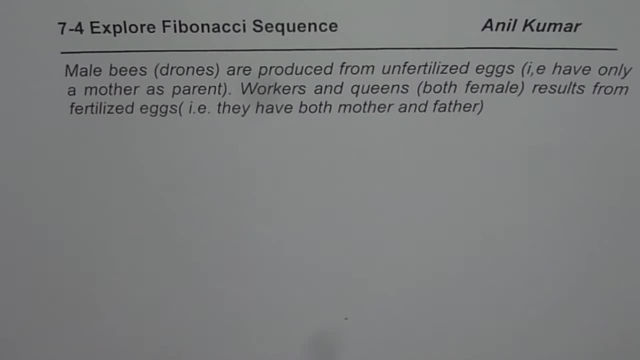 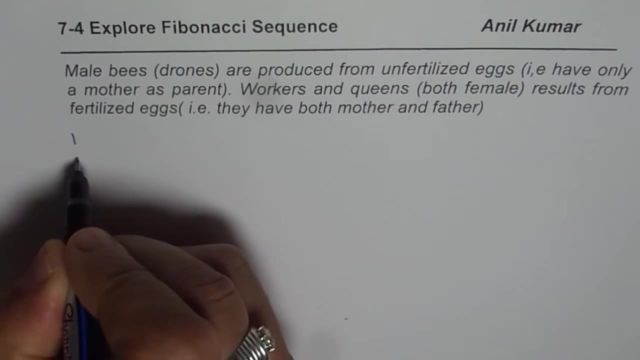 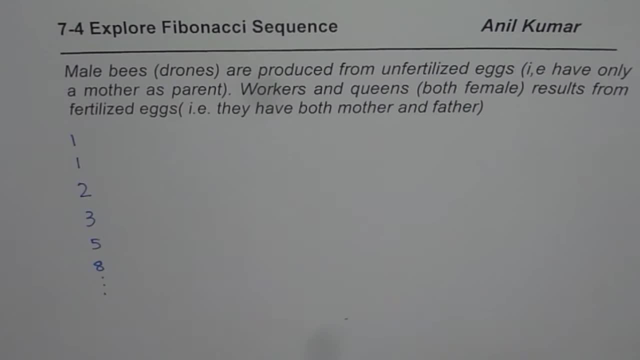 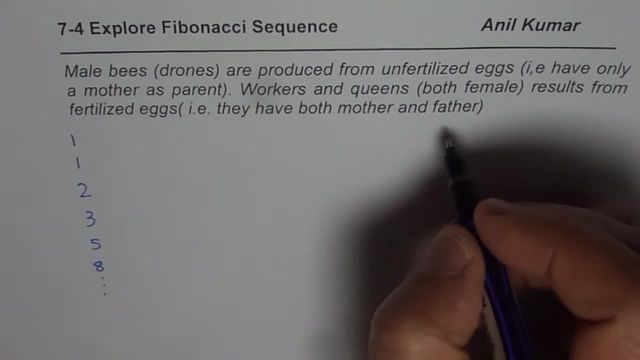 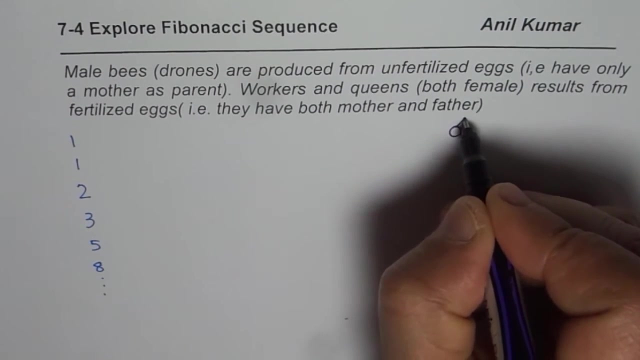 Now let us try to make a family tree for the Drones, So I will use 2 different colors. Let me use this blue color for Drones. So these are males, so we will use the symbol for males, which is this: 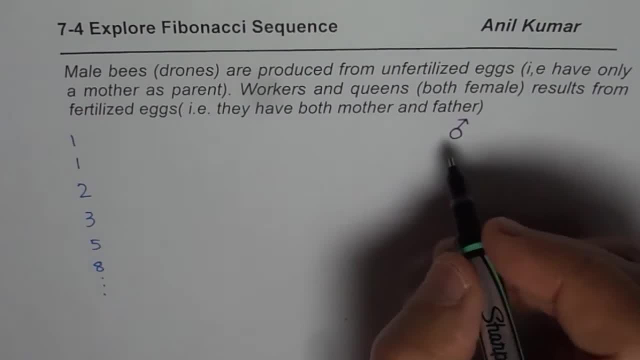 So that is a male. Now, a male will have only 1 parent, since they are produced from unfertilized eggs, And the parent will be the Queen Bee, So that will be a female, which could be written or shown with this symbol: 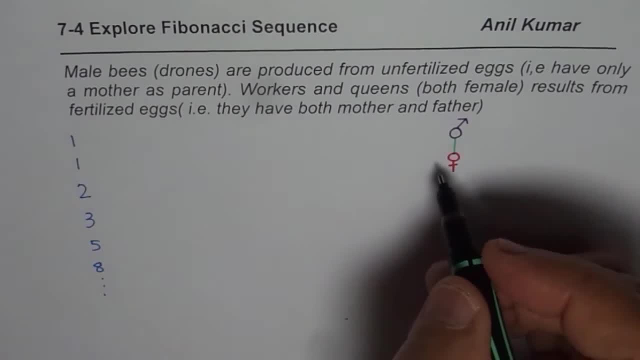 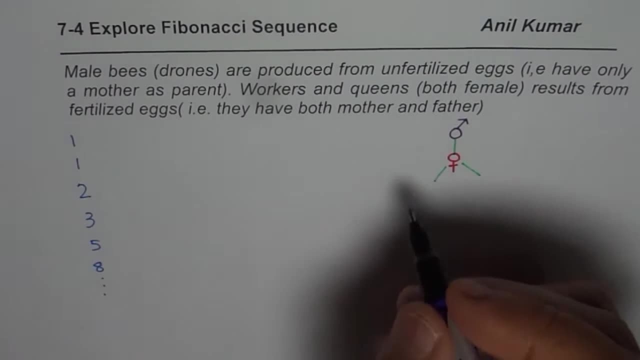 Perfect, Queen B will have both parents, right, Because these are fertilized eggs, correct? So Queen B will have a father and a mother, okay, So we'll put these symbols right there, carefully, right, And now again drones: the males will have just one parent. 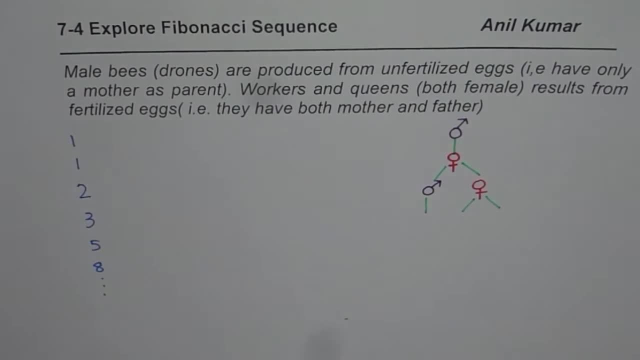 However, the Queen B will have two right. Okay Now, so the parent for the drone here will be again a Queen B. On the other hand, our Queen B will have both parents. So we have a queen and a drone. 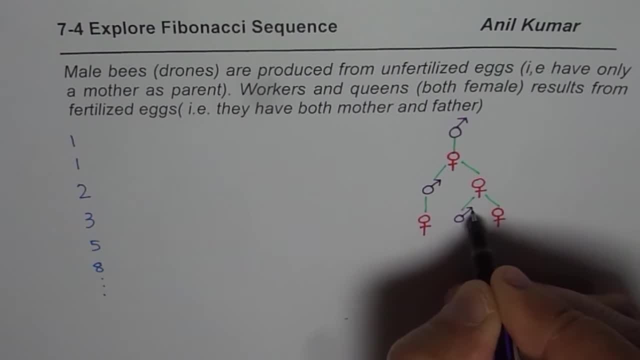 So let's continue. one more cycle Now. the female, the queen, will have both the parents as they come from the fertilized eggs. The male will have one and this female will also have two right, Both male and female parents. 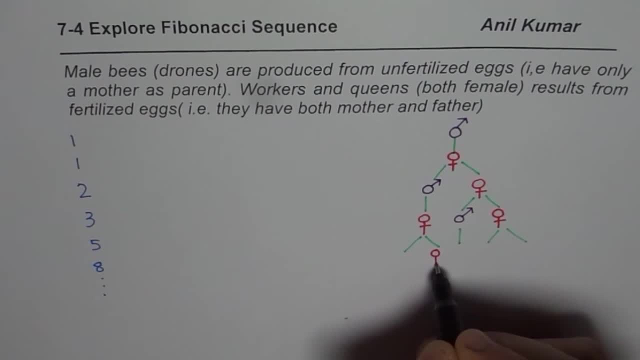 So we can show this as two. So that is it, And that's one, And this one. Let me, I should draw it here. It looks nice. okay, Now here we have a drone, right? Both parents, Both parents. 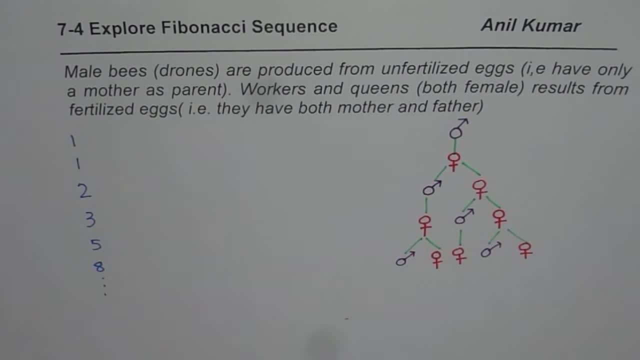 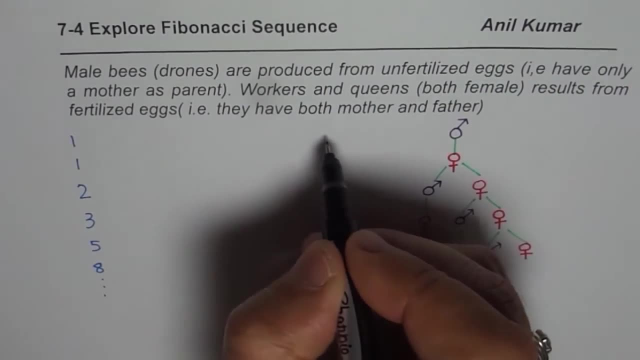 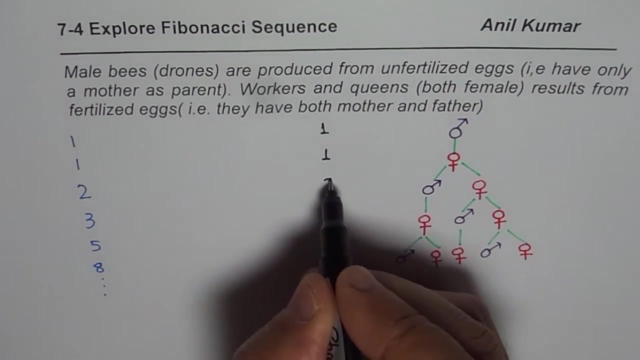 What do you notice? Does these numbers reflect something for you? Well, we started with number one, So number of Bs here is just one. In this case, it is still one. Then we have two of them, okay, And then we have three of them. 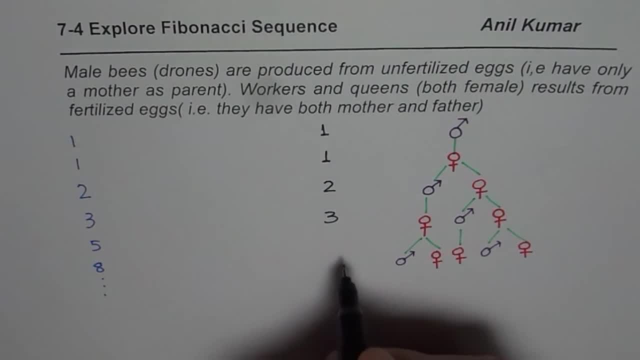 Fine, And then one, two, three, four, five, Perfect. So if you continue this pattern, you will actually produce the very famous Fibonacci sequence, right? So that is how it relates to so many things in the nature. So we'll do a couple of other examples also, but I hope you find it very interesting.